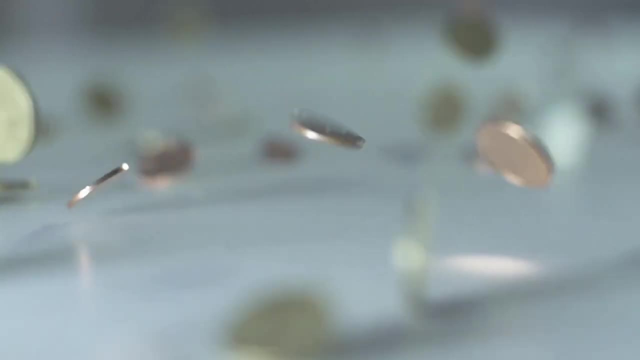 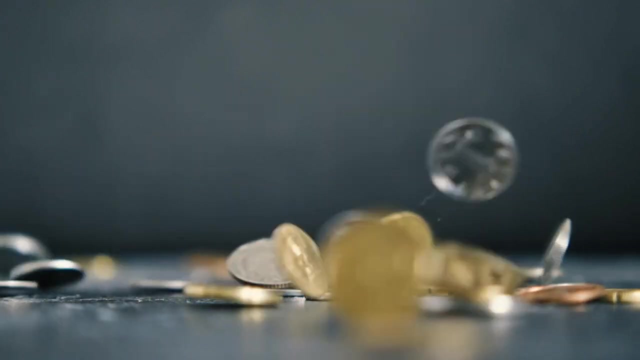 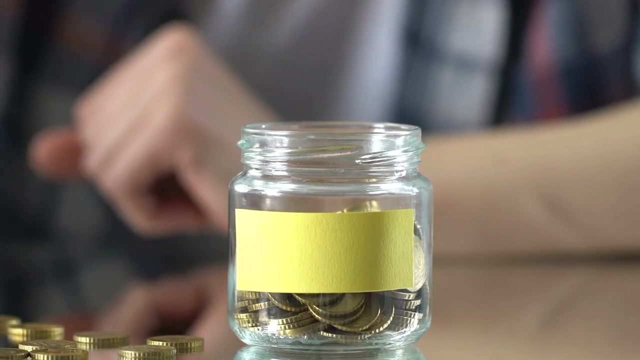 Someone bagged a five-figure sum for a single $0.25 coin And, if that's not interesting enough, more than 20 collectors showed interest in buying the quarter. However, this was no regular 1970 quarter. It had a unique error due to manufacturing issues at the San Francisco Mint, but more on that later. 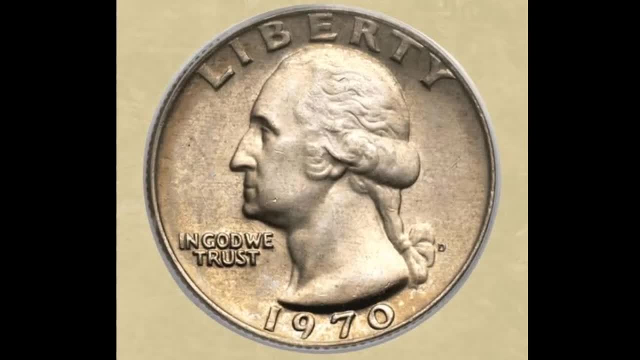 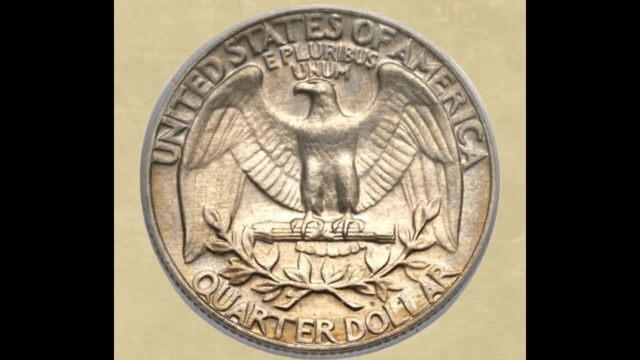 Whether you want to add a single rare 1970 quarter or complete your Washington quarter collection, you've come to the right place. Did you know? the US Mint introduced the first quarter in the 17th century, More specifically in 1796.. 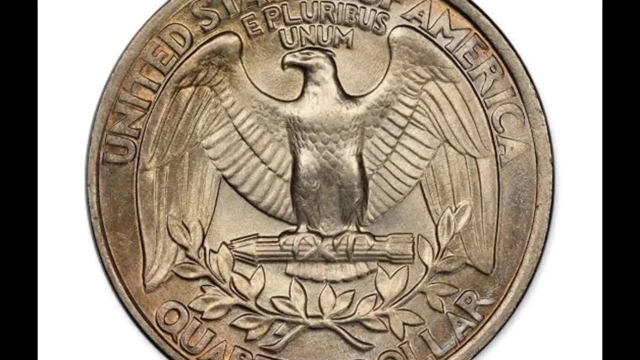 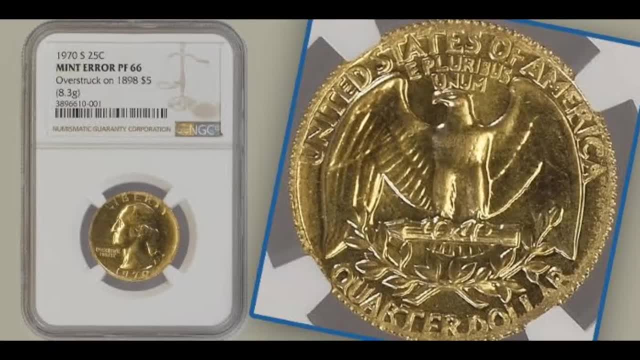 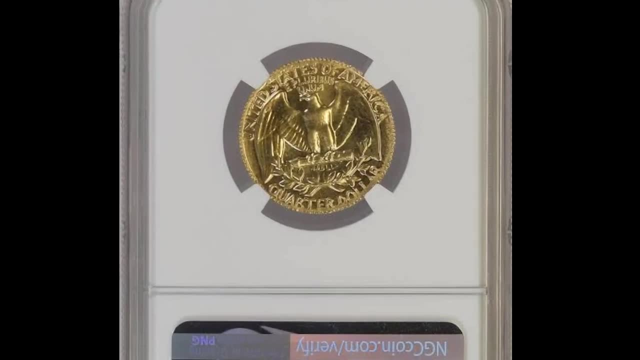 These quarters featured a bust of Lady Liberty on the obverse and an American Eagle on the reverse. The 1970 quarters, however, first entered circulation in 1932. At the time, the United States government was preparing to celebrate the 200th birthday of its first president, George Washington. 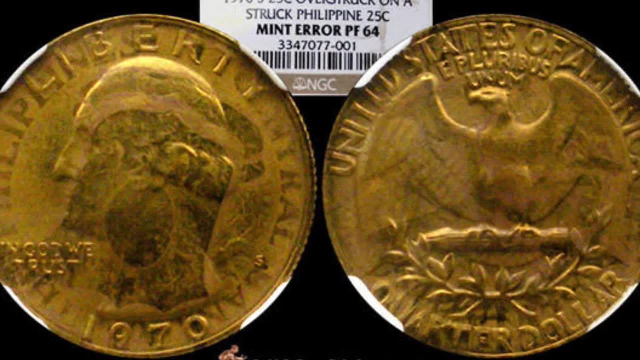 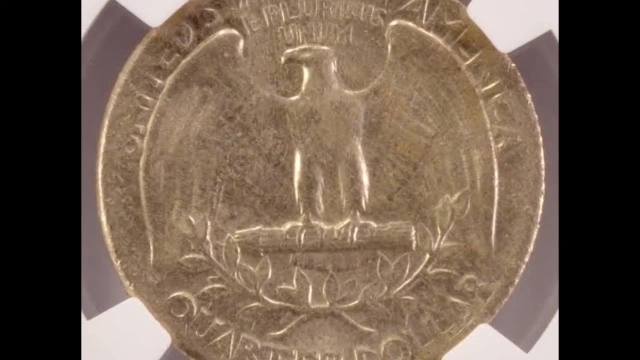 As a way of honoring him, the Bicentennial Committee established by Congress replaced the Standing Liberty Quarter with a new coin depicting Washington on the obverse, Hence the name Washington Quarters. Initially, the quarters comprised 90% silver and 10% copper. 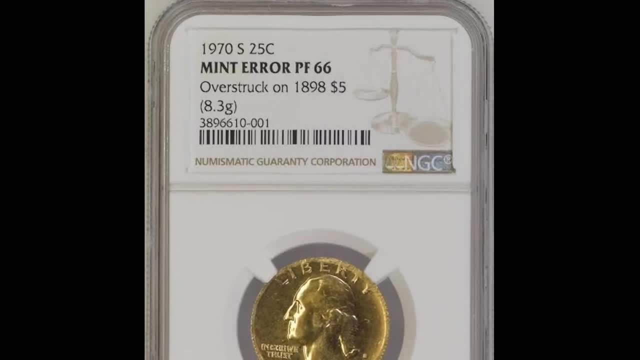 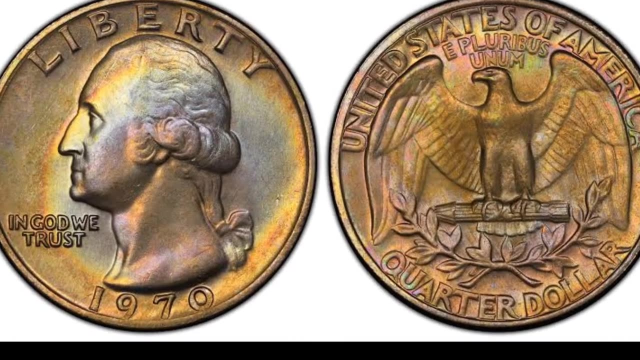 However, rising silver prices created a situation where the intrinsic value of the quarters exceeded their face value. This forced the Mint to adopt a new metal composition to mitigate hoarding and increased production costs. In 1964, the quarters adopted a copper nickel. 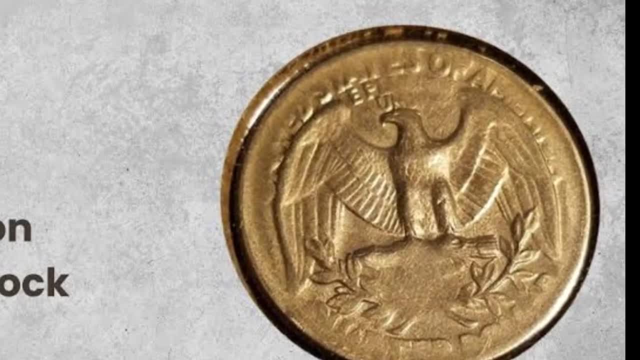 which made the coins more durable and practical. In 1970, Washington Quarters were minted in San Francisco, Philadelphia and Denver. In total, these centers produced over 500 million pieces, with the Denver Mint recording the highest mintage of $417,341,364. 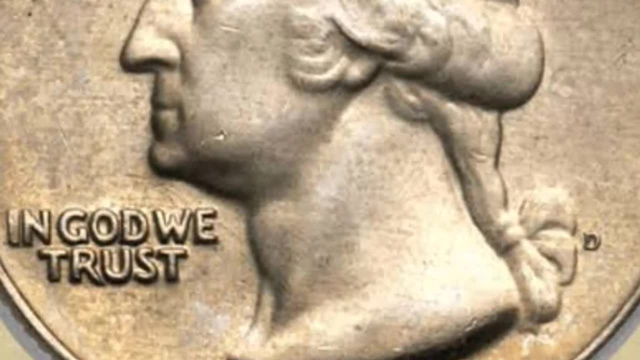 Well, the 1970 quarters are no different from modern-day Washington Quarters. They were minted in the 1970s, but they were also minted in the 1970s, in the 1970s, in the 1970s. 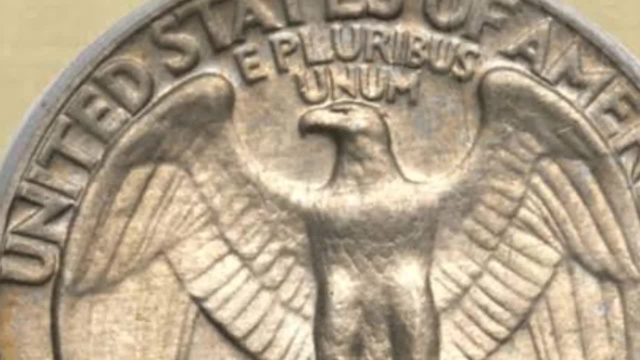 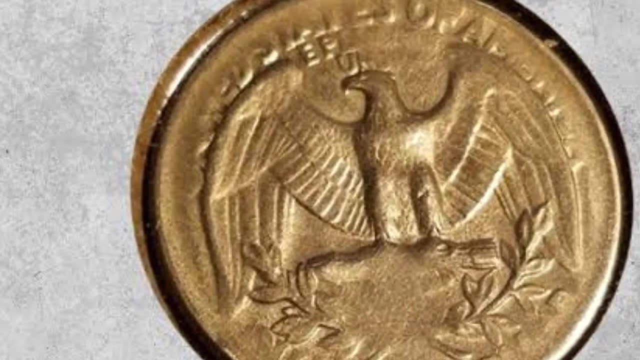 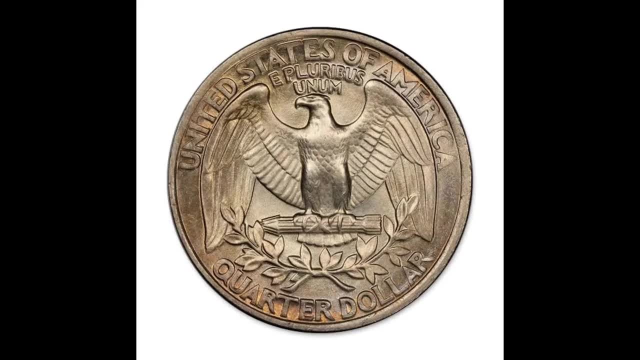 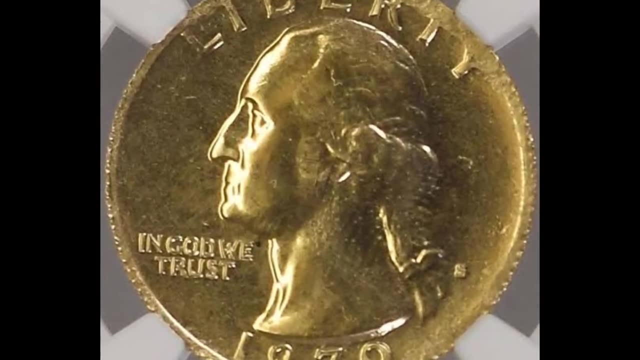 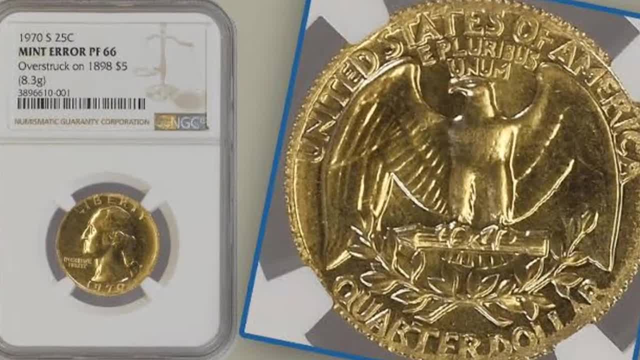 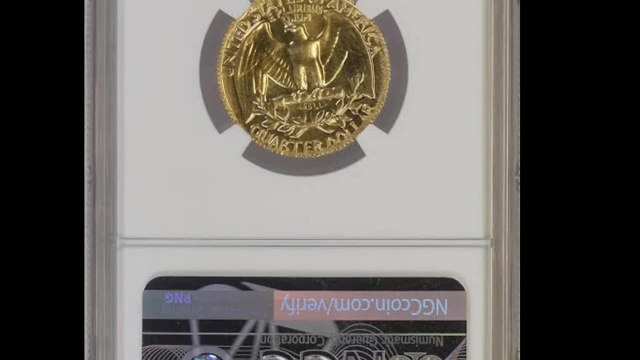 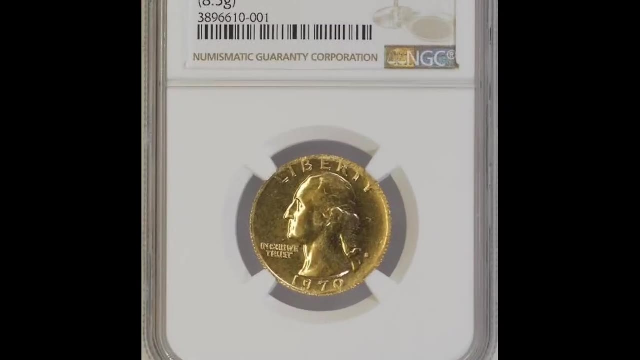 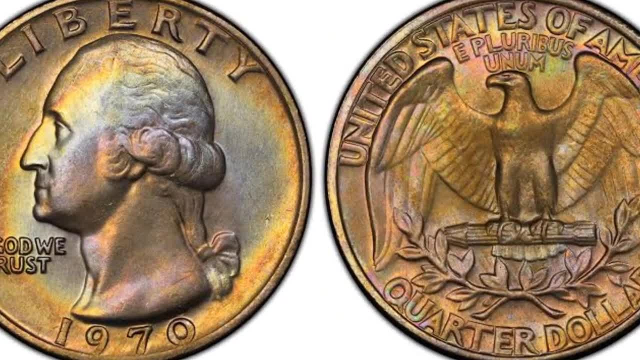 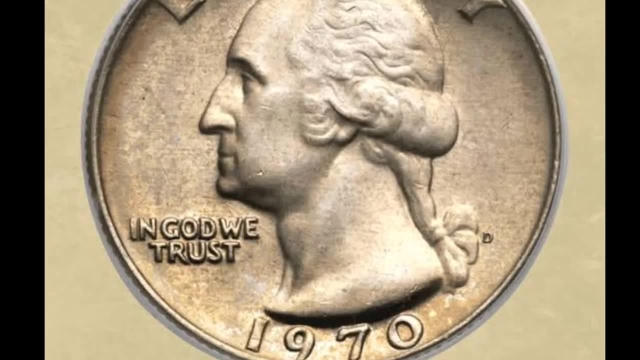 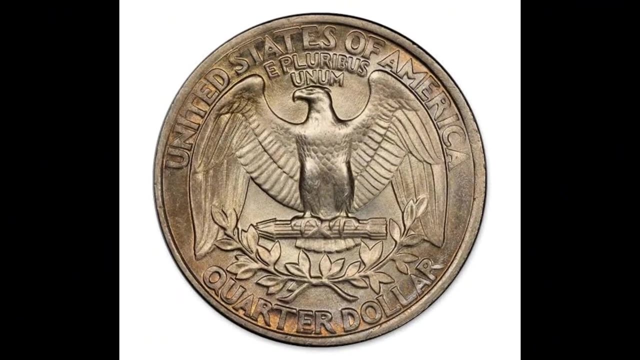 encircled by the words United States of America and quarter dollars. Additional 1970 quarter details. category: Washington Quarters Mint, Denver, Philadelphia, San Francisco. mintage 540,240,364. obverse and reverse design: John Flanagan. composition: outer layer: 75% copper. 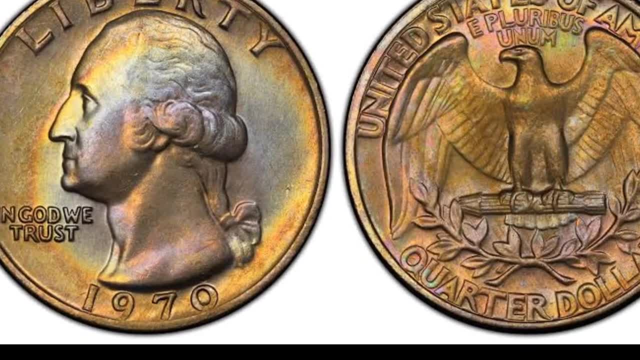 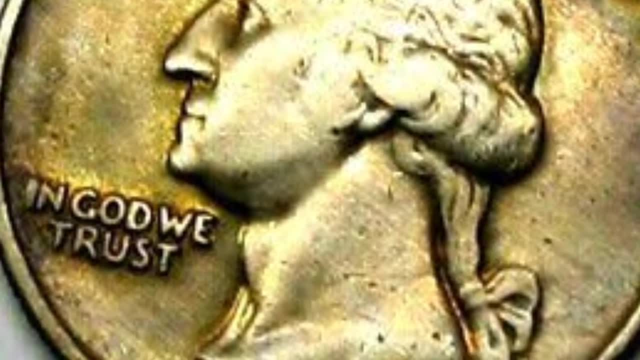 and 25% nickel clad core, 100% copper. weight: 5.67 g. diameter: 24.3 mm. edge reeded thickness: 1.75 mm. face value: 25 cents. As highlighted earlier, the Washington Quarters were minted. 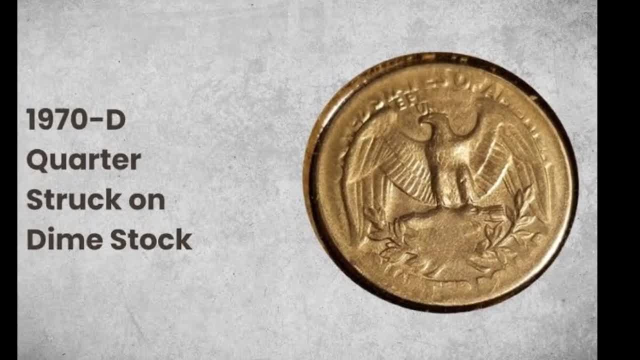 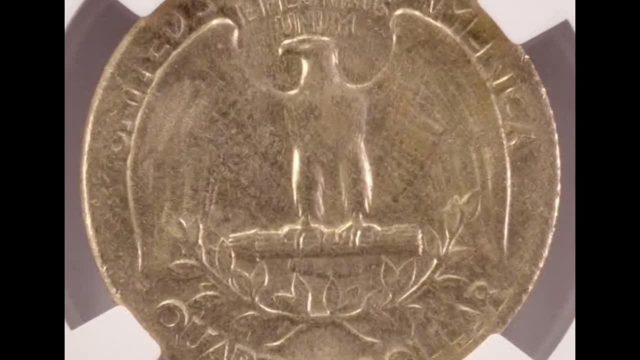 in millions in 1970 between three minting facilities. Therefore they are not rare. You can easily find them in circulation. You can buy uncirculated pieces from your local coin shop or online marketplaces like eBay. Of course, some quarters 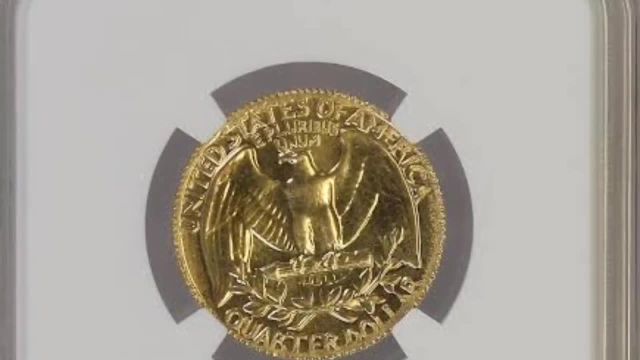 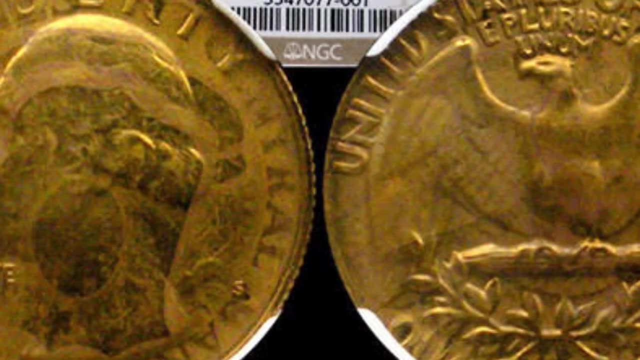 are worth far more than their face value of 25 cents, as you will see later in the article. But for now let's focus on the value of the regular 1970 quarter. Usually its value is influenced by several factors, including mint marks, conditions and errors, For example. 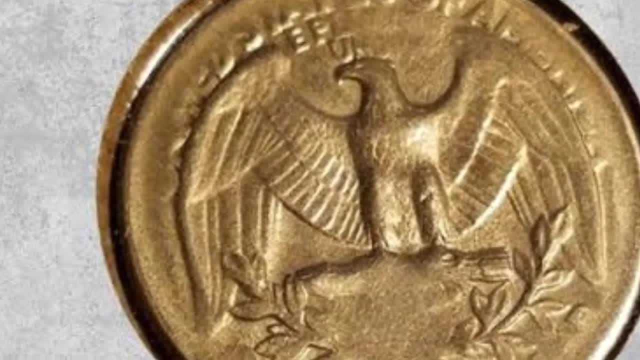 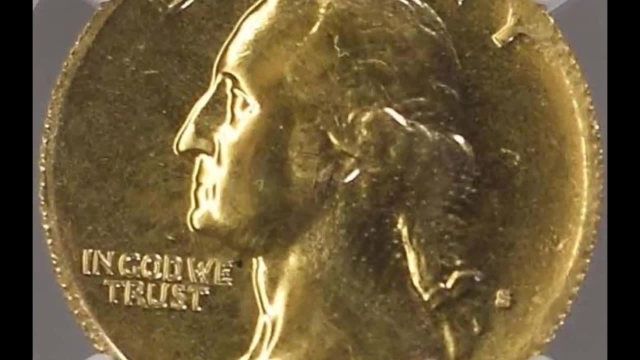 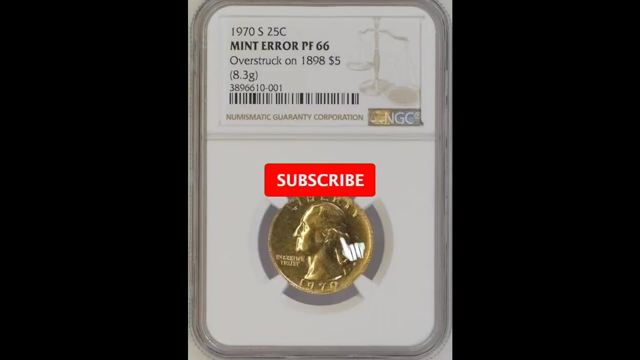 quarters struck in the Philadelphia mint in 1970 cost no more than their face value. However, pieces from Denver and San Francisco mints might have a higher value depending on their condition. In terms of condition, a circulated 1970 quarter is worth anywhere from 50 cents to $1.. But as the quality of the coin improves, 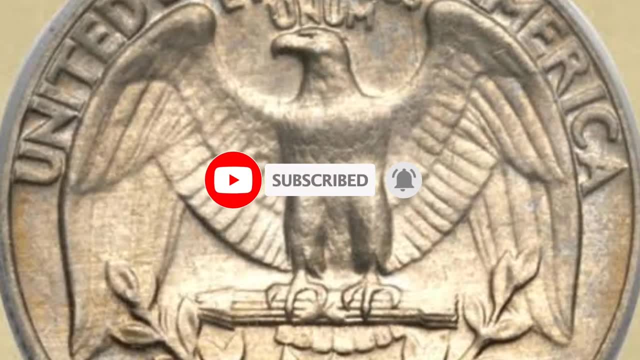 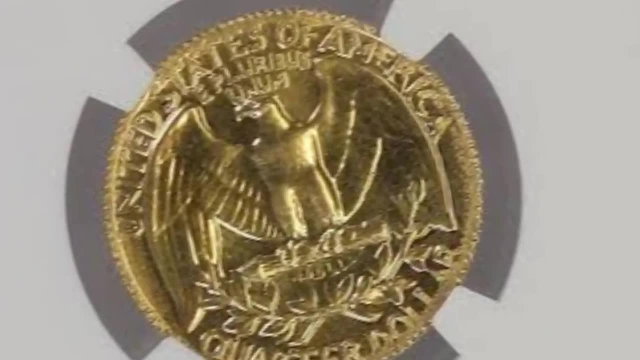 so is its value. So if you have discovered an uncirculated sample from your grandmother or grandfather's coin stash, you may get $1.20 or more for it. However, examples with a high-grade mint stash are not as valuable as the quality of the coin. So if you have discovered an uncirculated